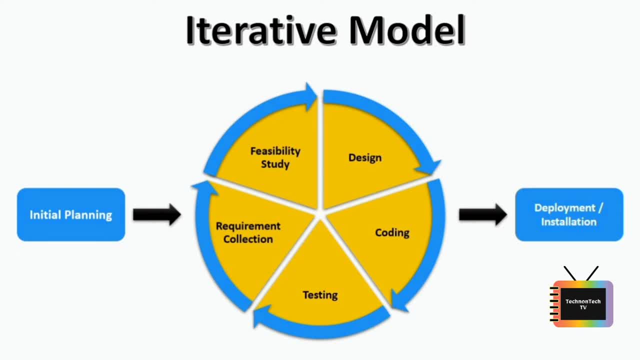 the overall end product is improved and iterated on. These stages are repeated if any new requirements popup or any error bug is identified in our system. So once these stages are finished- in other words, all the requirements are fulfilled and checked- The most recently built iteration of the system is given to the end user. 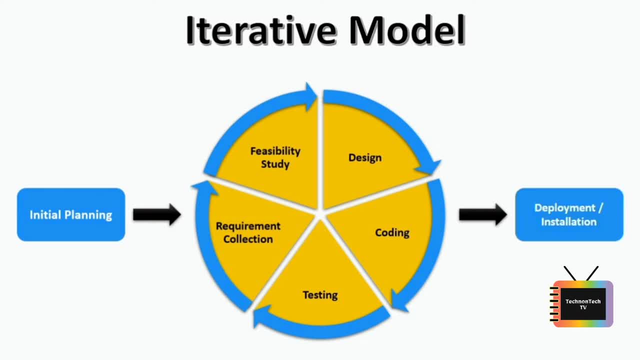 This model iterates planning, design, coding and testing stages again and again. This helps in ensuring that the final product build iteratively is according to the standards required by the user. So I have already explained all these stages in detail in the previous video. that is waterfall. 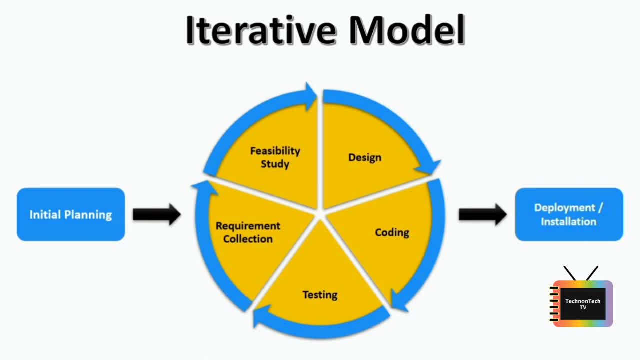 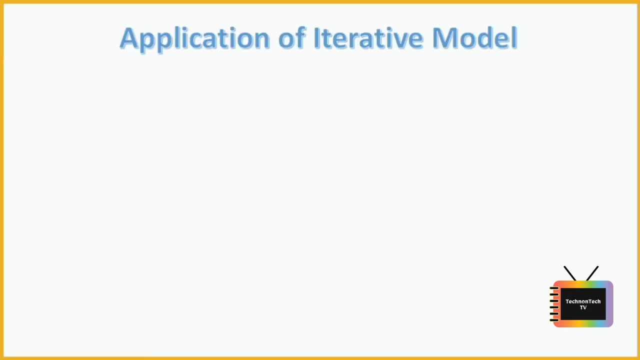 model tutorial. So if you want to know more about these stages, then watch that video first. I have added the video link on the upper right corner of your screen. Now let's discuss application of iterative model. So the iterative approach is used by many engineering teams to develop new features. 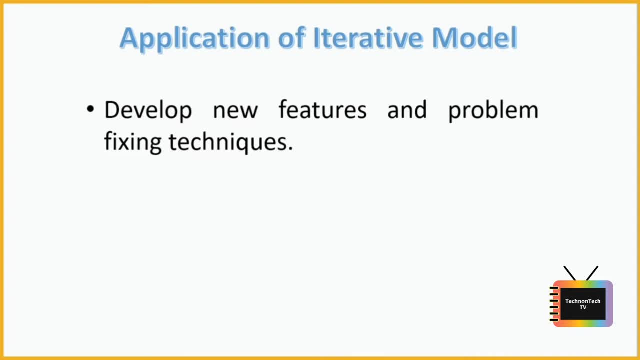 and apply problem fixing techniques. So the team may frequently produce new iterations that they believe are equally promising, before testing them with users. So they will make a list of pros and cons and then work on the one that perform the best. So this process is then carried out in a loop until the results are satisfactory. 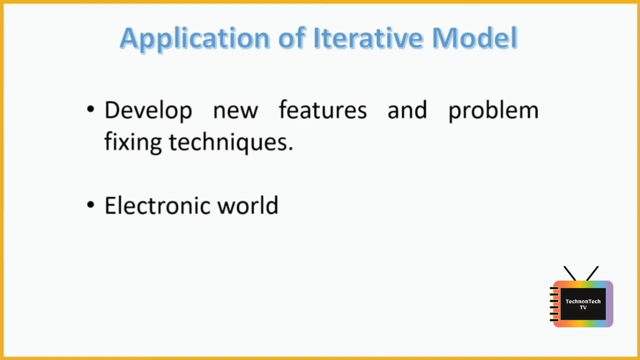 This model is also used in electronic world. So the world of electronics is following the iterative model: The development of mobile phones throughout the years, how speakers have gotten smaller and more portable over time, or even the way refrigerators from the same brands have changed. 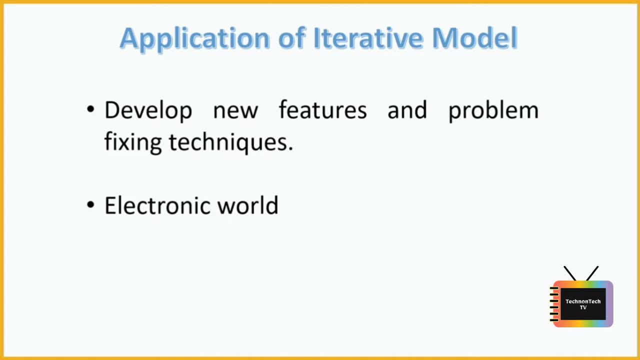 to adapt to new family needs. So all of these are iterative processes. The industry is reshaping itself every day based on customer feedback. Next is digital marketing. So the digital marketing teams test different advertising strategies to see which one gets better engagement. So they understand the requirement of the advertisement plan. attractive designs by 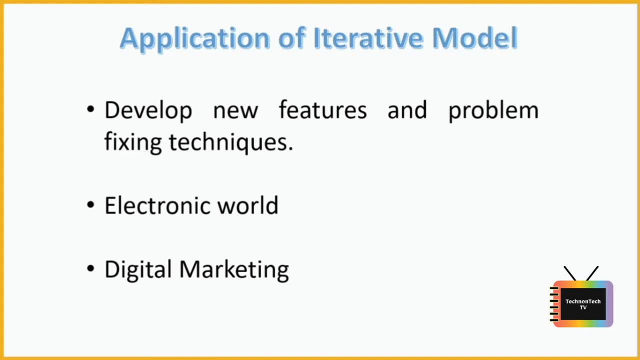 performing proper analysis and implement them in their product marketing. So these copies are then shared with the members to get feedback and based on that the improvements are made. So this improves their marketing strategies. The use of an iterative model does not limit to one industry.